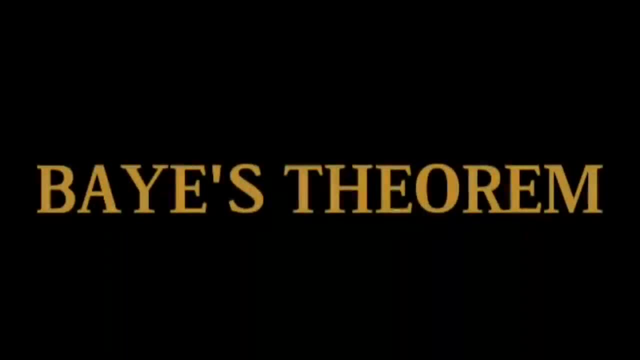 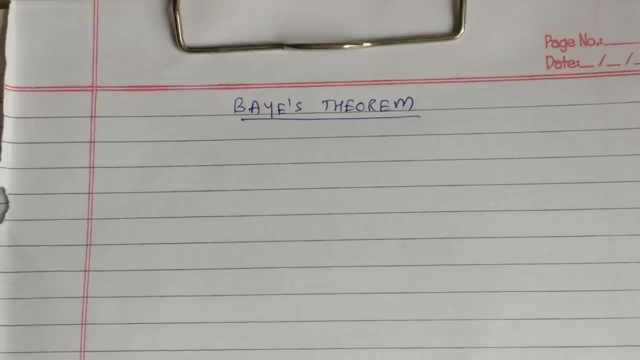 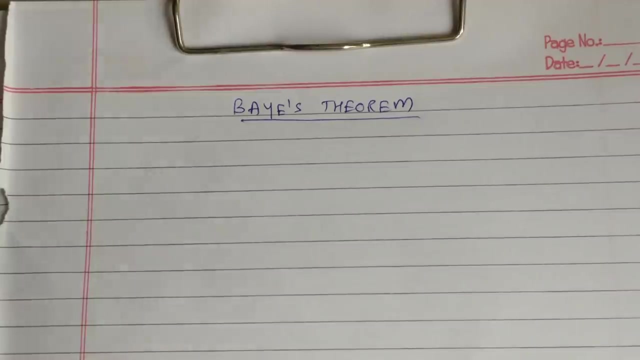 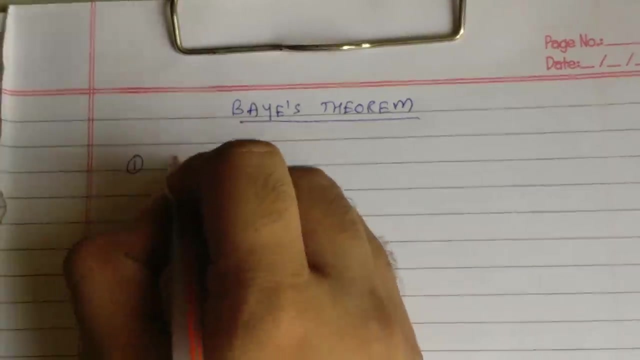 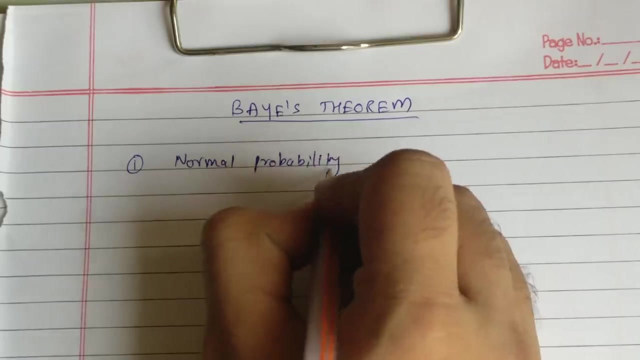 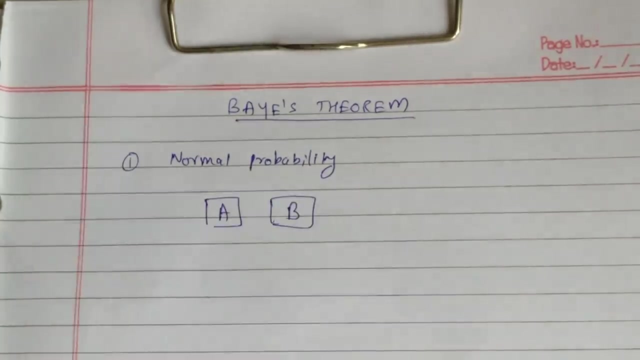 Hey guys, if you want to solve Bayes Theorem questions in less than 30 seconds, please follow the following instructions. First thing that you should know is about normal probabilities. So what are normal probabilities? It is like if there are two boxes, box A and box B, So what is the probability of selecting box A? So it is represented as 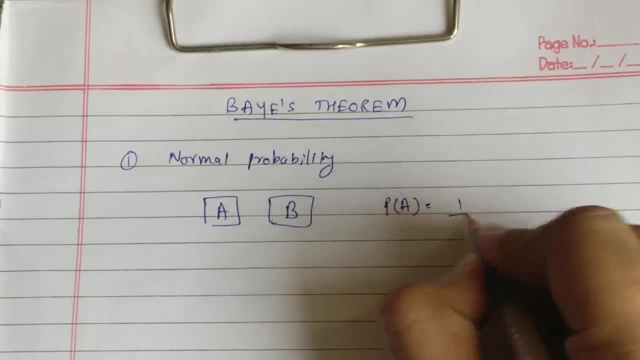 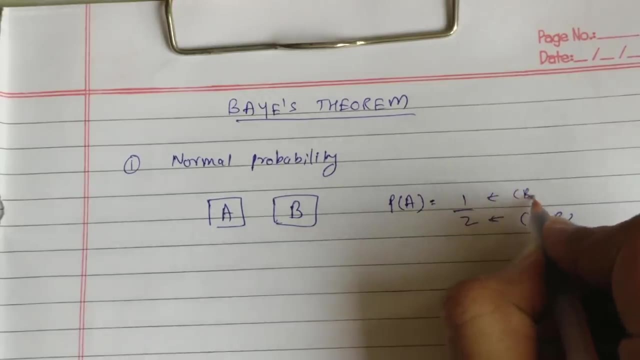 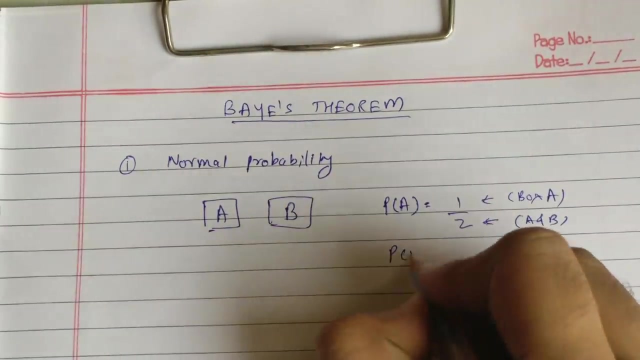 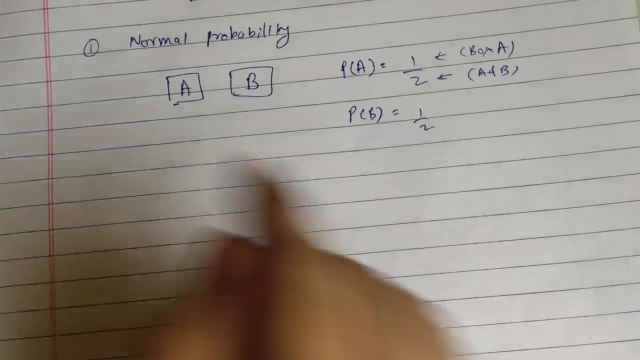 probability of A that is equal to 1 by 2.. So how 1 by 2?? There are two boxes, A and B, And we have selected the box A. Similarly, if we have to select the box B, the probability should be- probability of box B- equal to 1 by 2.. Now consider next case. If there are 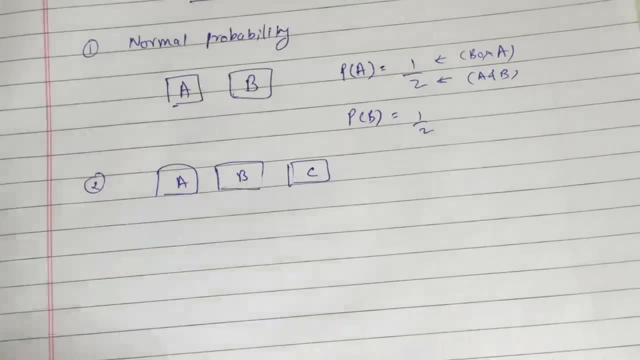 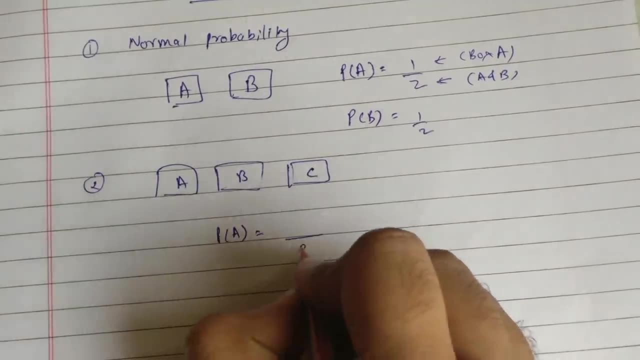 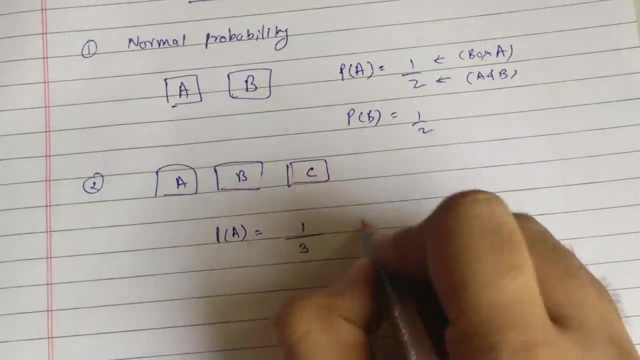 three boxes: A, B, C. So what is the probability of selecting box A? So we have to select box A. Total number of box: 3.. So we have to write in the denominator 3. And we have to select box A And there is only one box A. So 1.. Similarly probability. 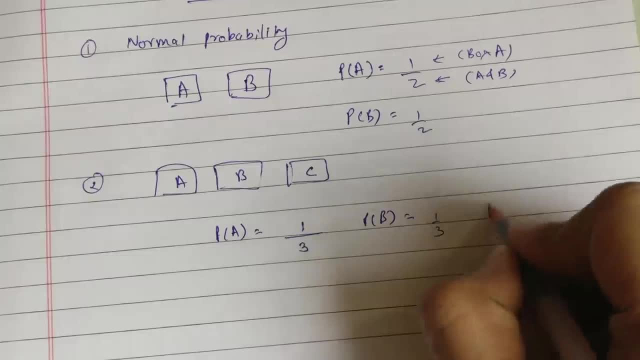 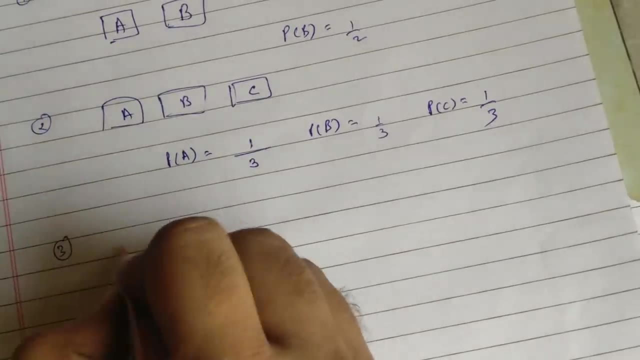 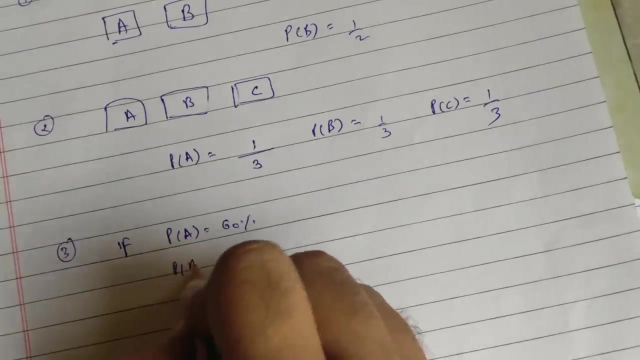 of box B equal to 1 by 3.. And probability of box C is also equal to 1 by 3.. What if they have given in the question the probabilities of individuality? So if P of A is given as 60 percent and P of B is given as 30 percent and P of C is given as 10 percent? So you 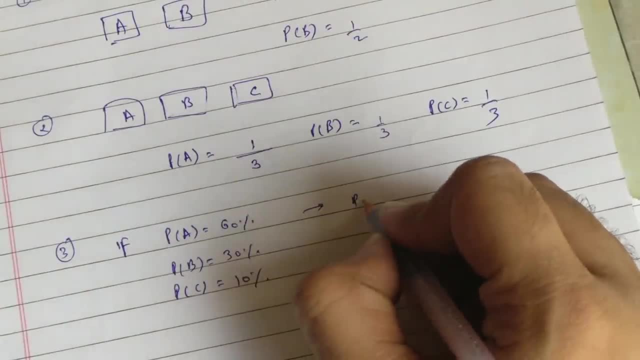 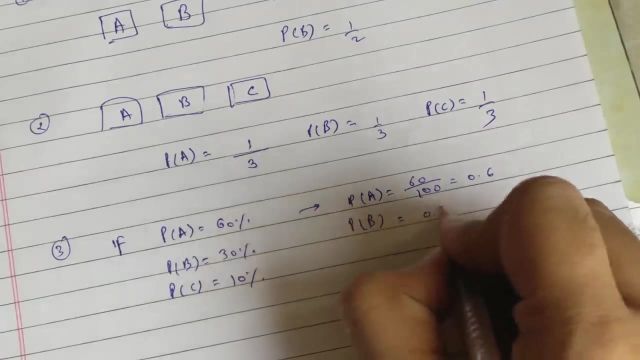 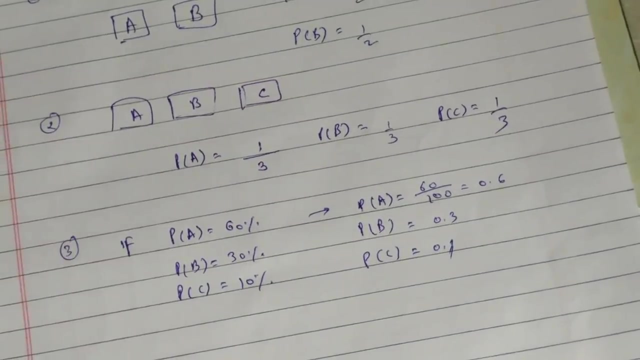 have to convert this percentage into fraction. So P of A is equal to 60 by 100, that is equal to 0.6.. P of B is 0.3 and P of C is equal to 0.1.. So you know the first step, that is. 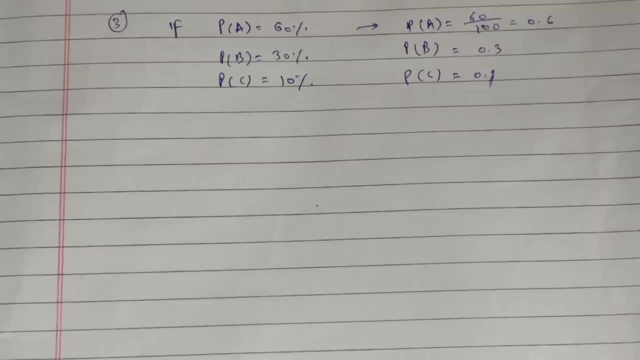 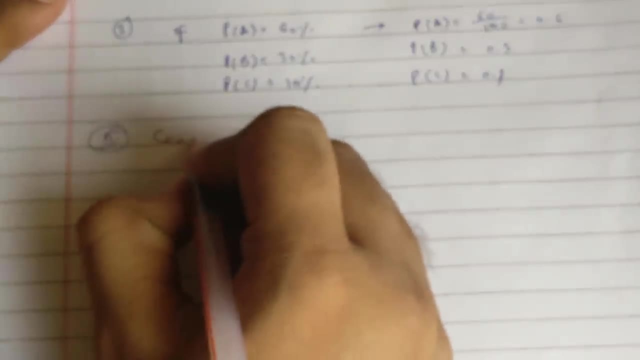 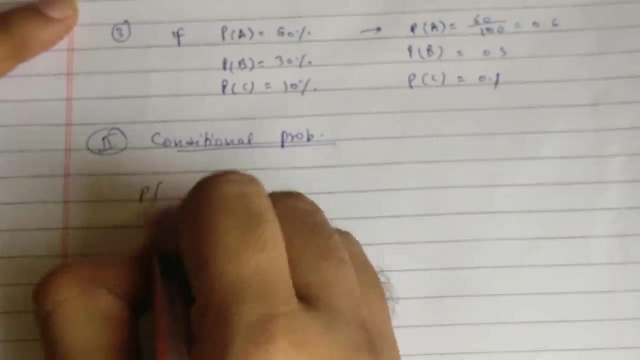 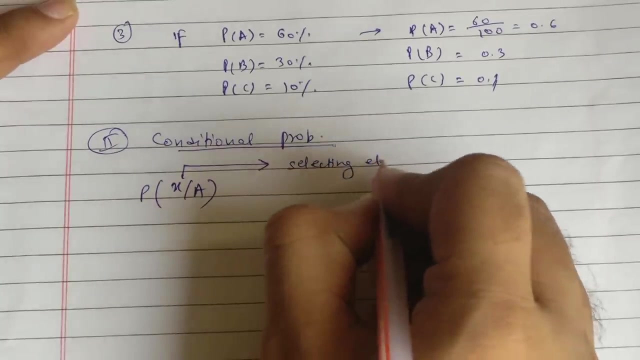 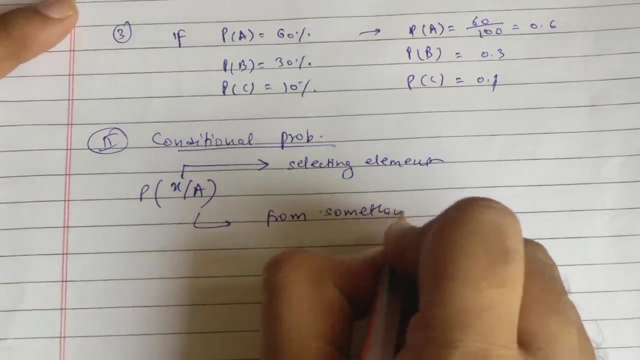 to find the normal probabilities. So the second step is about conditional probabilities. So, conditional probabilities, It is represented as X over A. Now the meaning of X is selecting elements And A means selecting elements from something. Let understand this by an example. Suppose we have a box A And 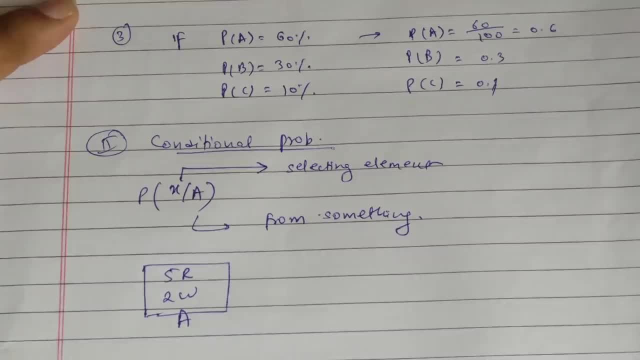 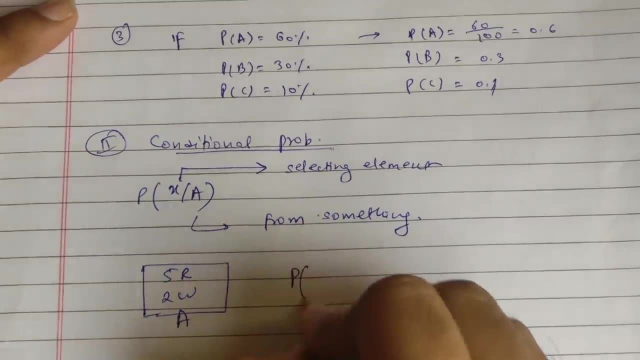 the box A has 5 red balls and 2 white balls. So if we have to select a red ball from this box, what will be the probability? So we have to select red ball from box A, So it is a conditional probability. The answer should: 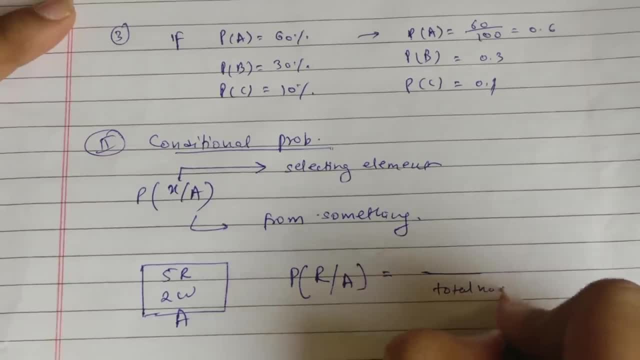 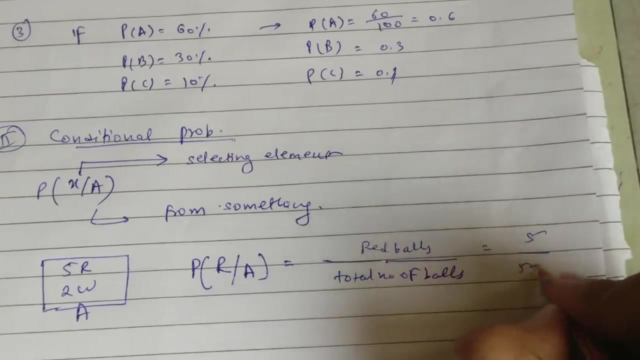 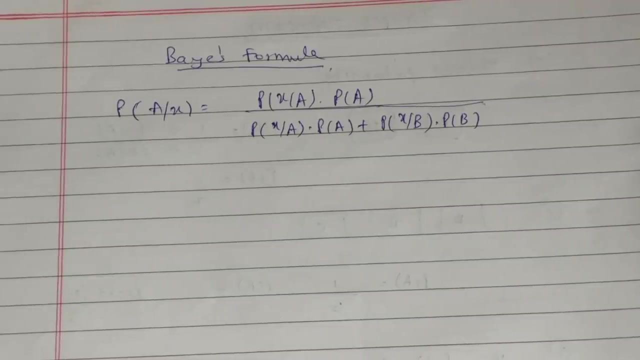 be total number of balls at the denominator and we have to select red balls. So upper should be the red balls, So answer should be 5 red balls. On the other hand, the third step is the base theorem. So the base theorem is this This: 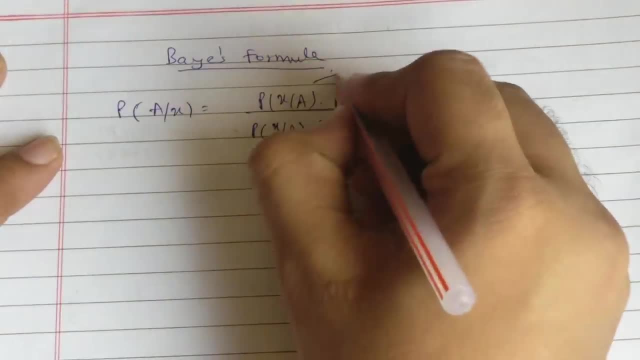 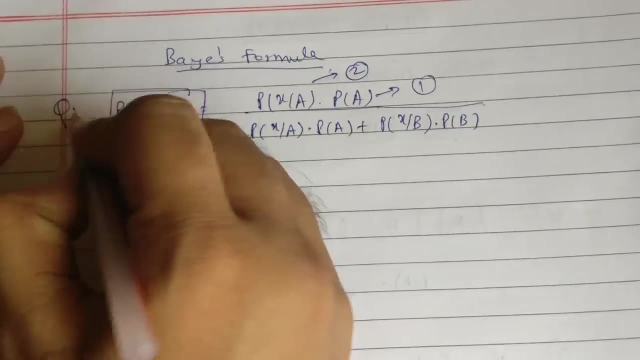 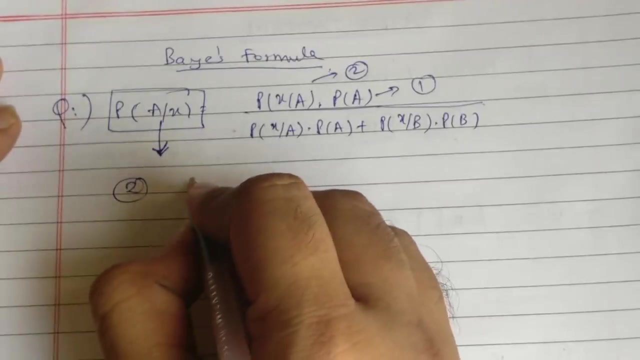 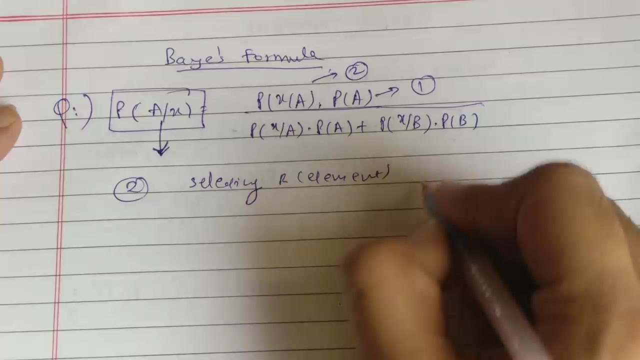 is our first step, the normal probability. This is our second step, The conditional probability, And the question will be to find this Now. what does this mean? This means the second step meant was selecting elements, red or something element, selecting element from box. so the question will be: 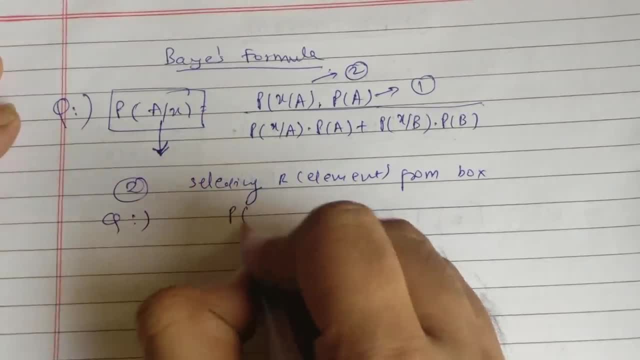 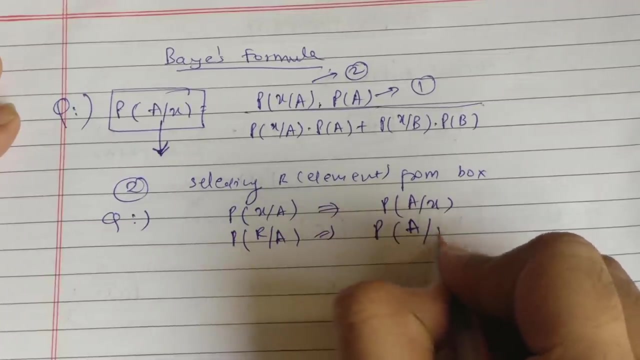 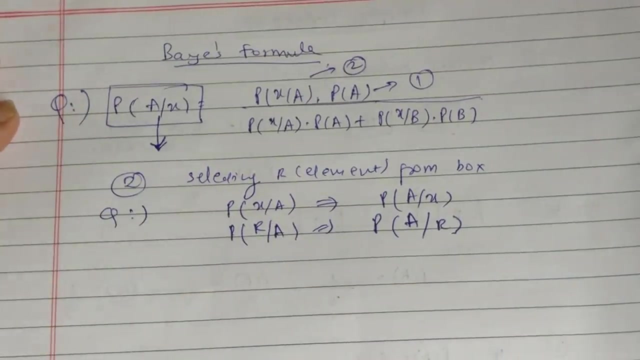 the opposite, exactly opposite of that. suppose we have P of X over a, the question will be P of a over X. if we have P of red balls over box a, then the question will be box a having the red balls. so we have to solve the straightaway example to understand the concept clearly. the standard question: 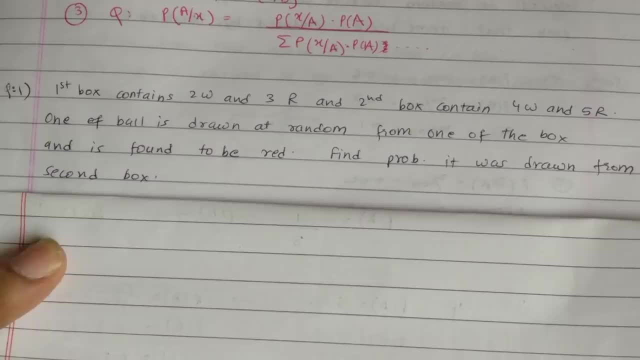 let's read the question. the first box contains two white and three red balls, while the second box contains four white and five red balls. one of the ball is drawn at random from one of the box and it is found to be red, find probability that it was drawn from the second box. now your task is to find the first step. 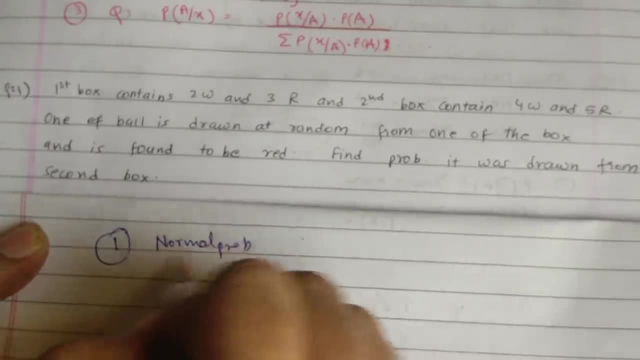 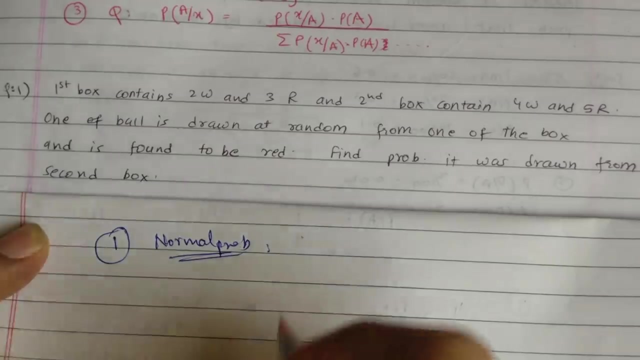 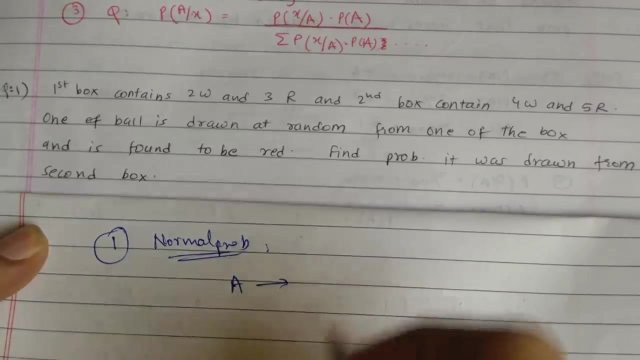 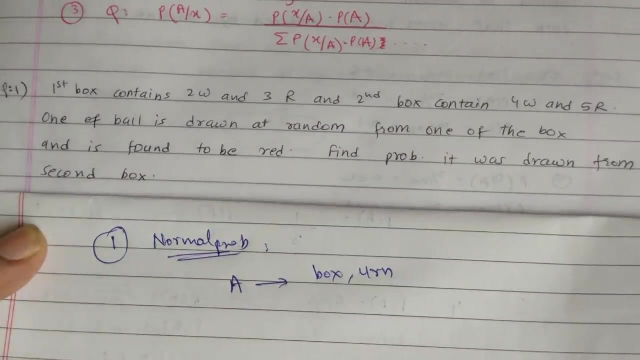 that is the normal probability. here we have to consider what should be a. now here is the trick. a should be that value that has the element, like. it should be box, or it should be an somewhat like that. you should be that, something which has the element, so in. 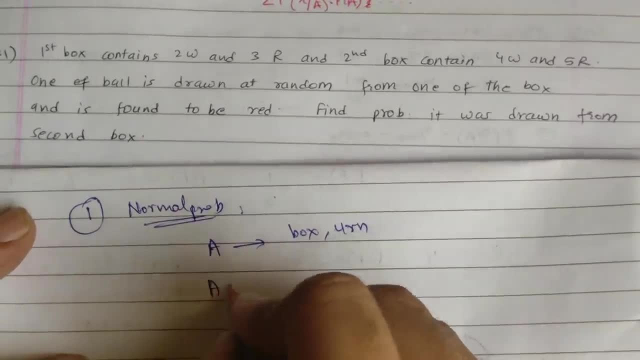 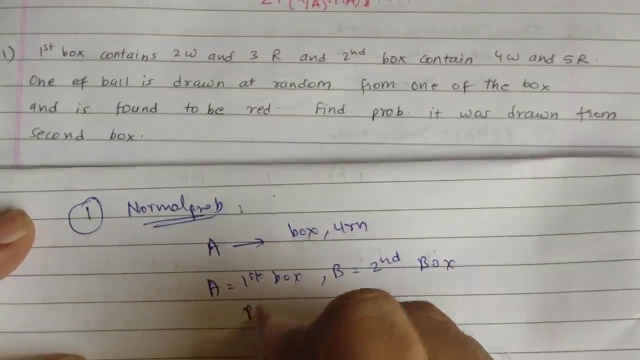 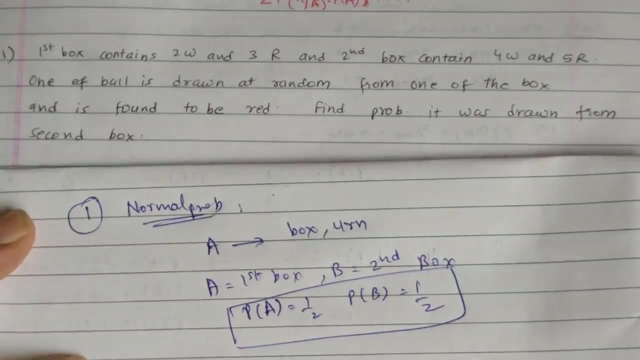 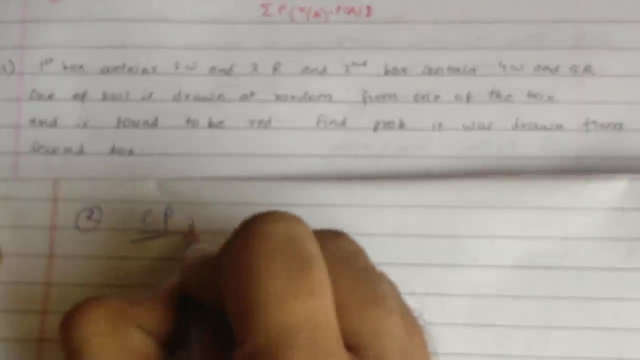 this case our A is equal to first box, while P equal to second box. so probability of a equal to half and probability of B equal to half. so we are done with step one. now comes the step two. step two: now comes the step two. 2 is conditional probability. here our x and y are different. we have to understand the question. 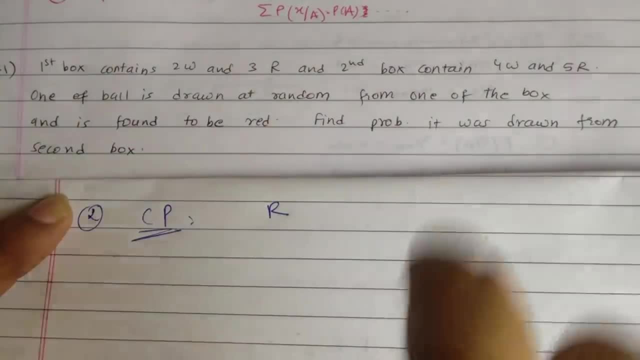 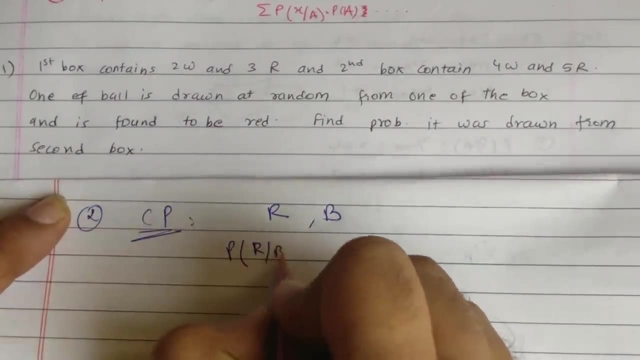 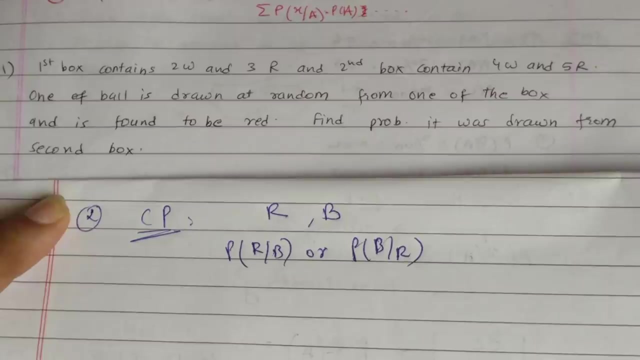 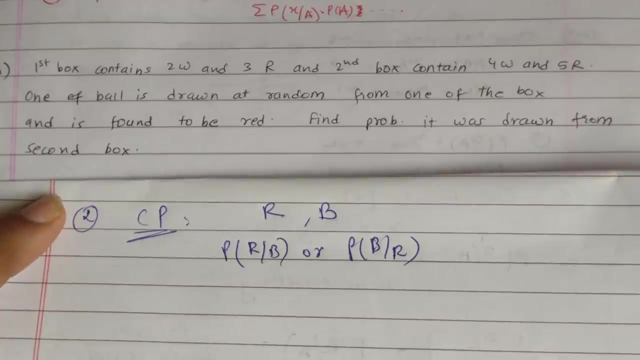 they want red balls and it should be drawn from second box. so probability should be red over b or p of p over r. you are confused in that, so you have to understand it very clearly. now. what you know is the real question. do you know that there are some? 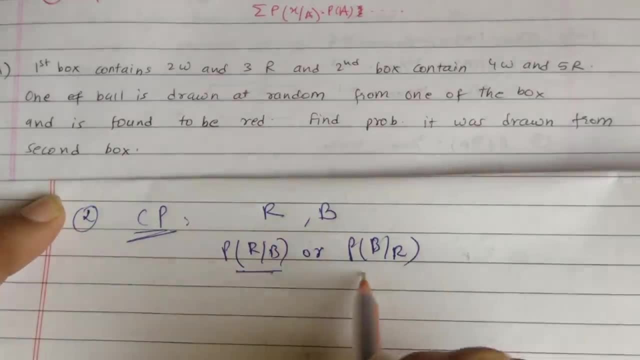 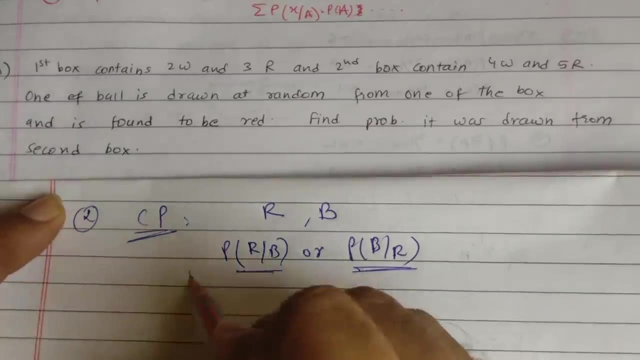 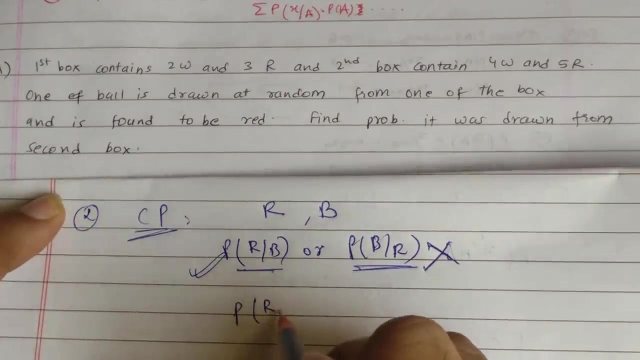 red balls in a, in box b, or you know that b has some red balls, is a confusing kind of thing, but you should be sure that you know this. and you don't know this how, because we already studied that we can select red ball from some box, so red. 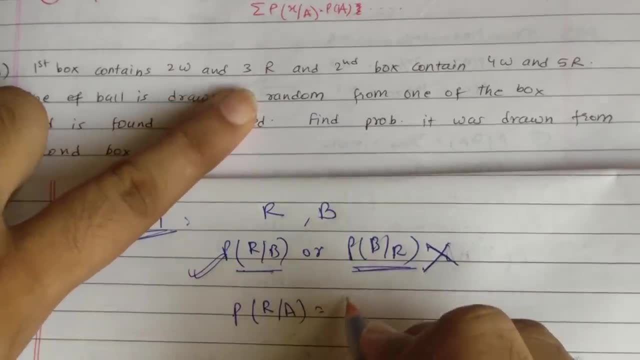 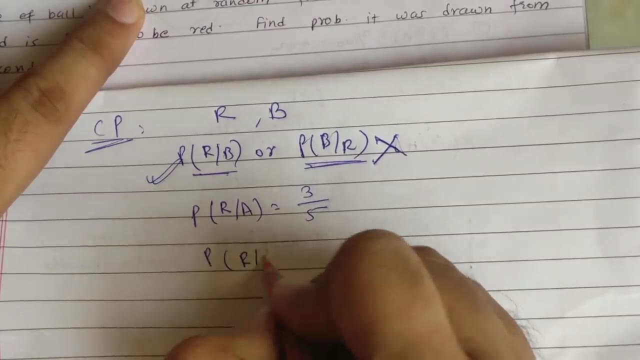 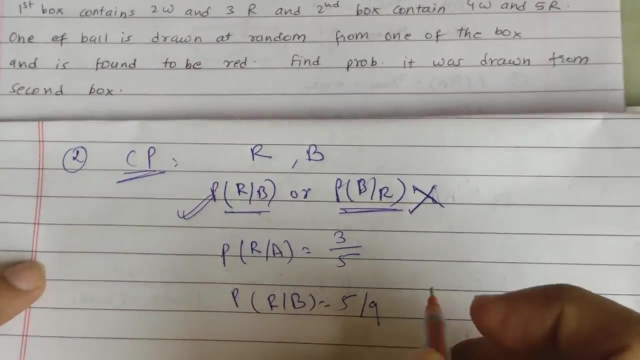 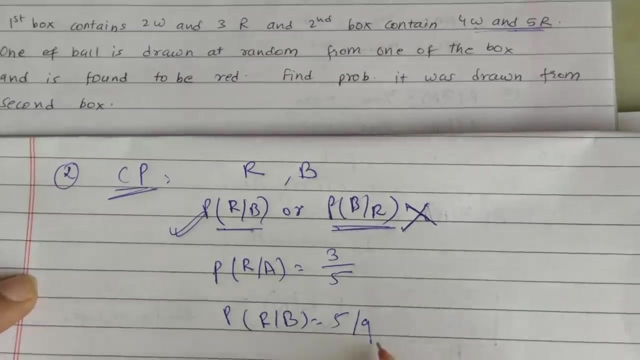 ball from a box will be 3 over 5 and probability of red balls over b will be equal to 5 over 9. it is clearly mentioned that there are total 9 balls in box b or in second box, you can say so. total is 9 and there are 5 red balls. in box a there are 3 red 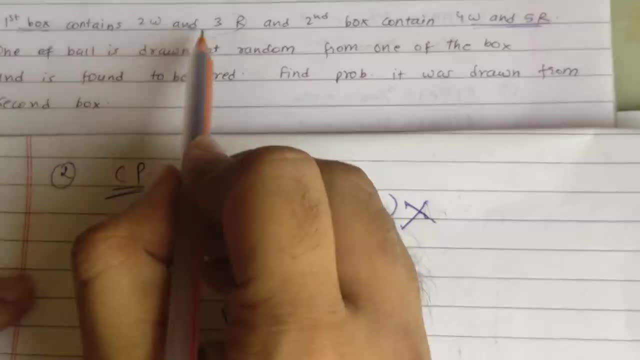 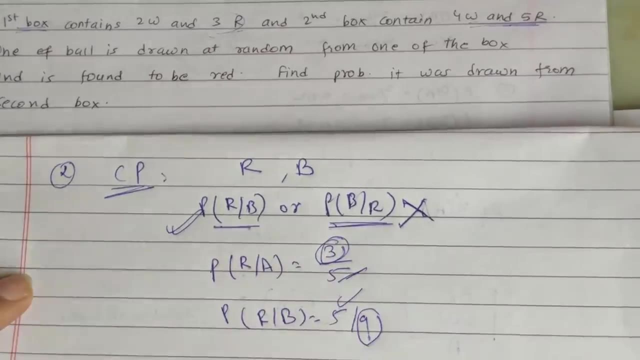 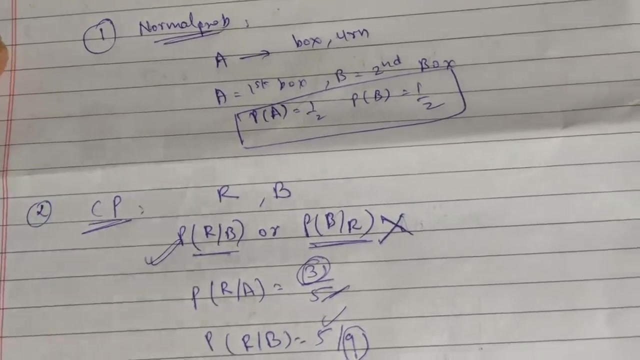 In box A there are 3 red balls, so we have to take R. here is 3 and total is 5.. So we have done our first step, that is normal probability, and our second step, that is conditional probability. So what we have now, we have to write that perfectly. 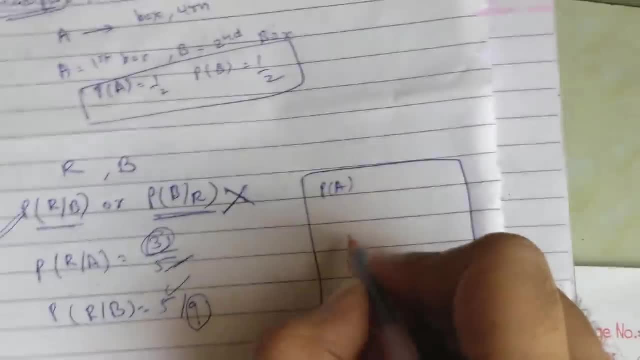 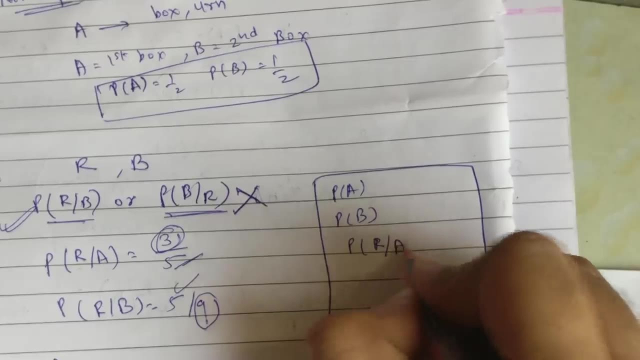 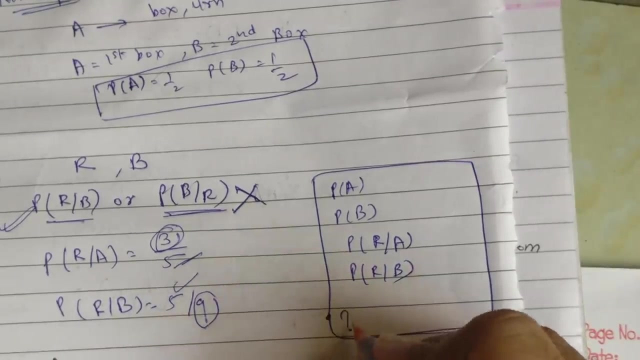 We have P of A, we have P of P. we have P of A, we have P of P, we have P of R over A, we have P of R over P. All right, now we have to find the question. what is the question? let's jump to the question. 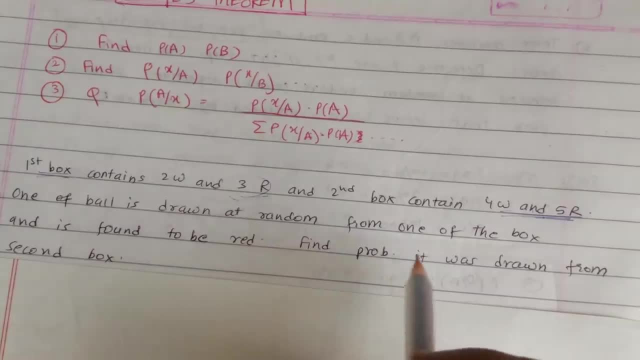 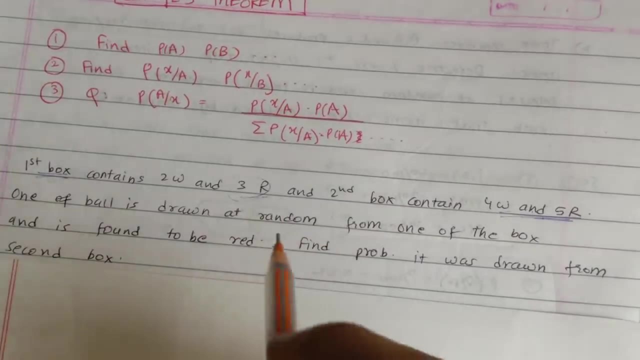 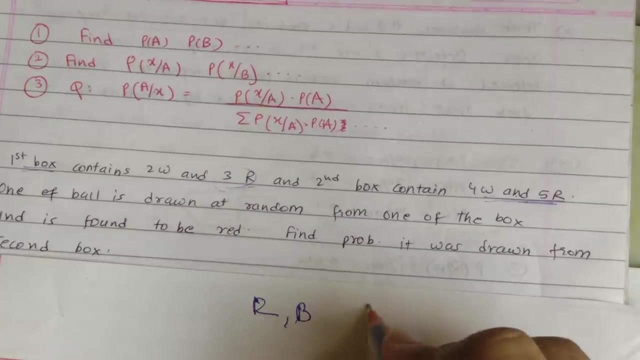 The question is: one of the ball is drawn at random from one of the box and is found to be red, So red is mentioned in the question. find probability. it was drawn from second ball and we know that it is from second ball. So we have already found P of R over P. so question cannot be this. the question should: 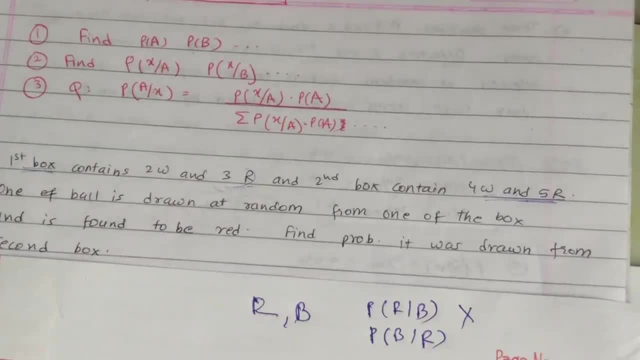 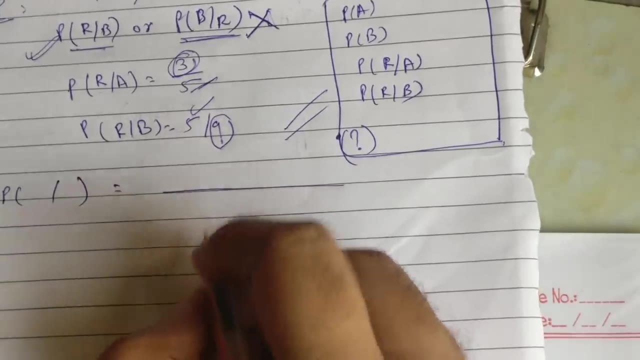 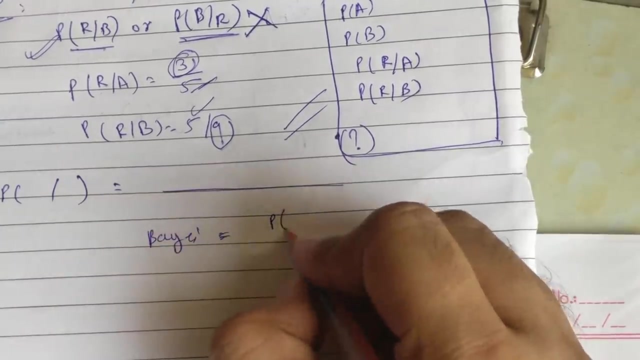 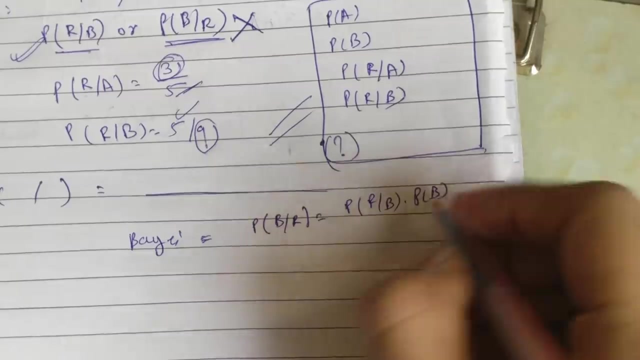 be opposite of that: P over R. Apply the formula. we have all of this now. apply the formula according to the base theorem. according to the base, The formula should be like this: The question is this: P of B over R. so formula is P of R over P into P of P upon P of R over. 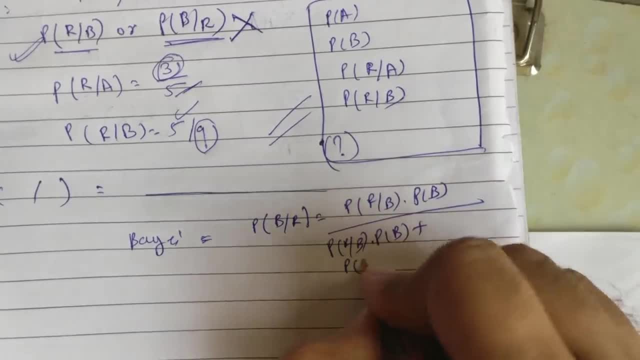 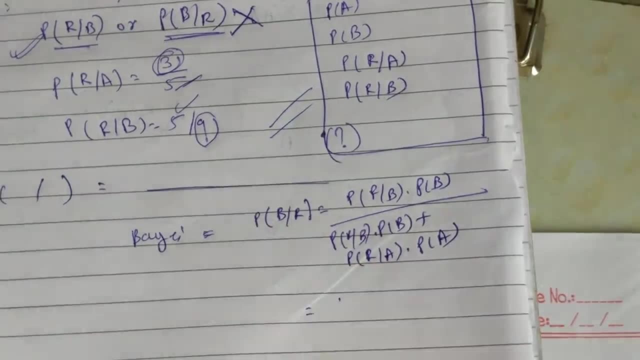 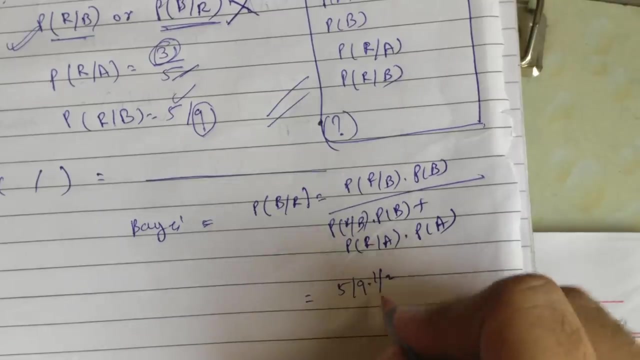 B into P of P plus P of R over A into P of A. So just plug in the answers and you will get answer like five by nine into one by five by nine, One by two upon five by nine into one by two, plus three by five into one by two. 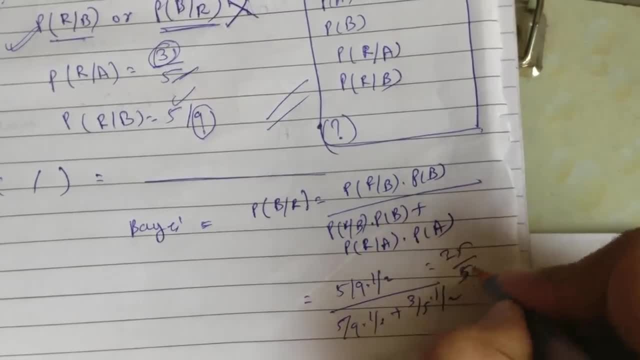 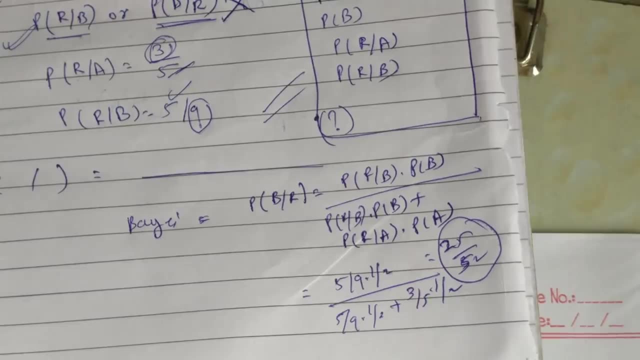 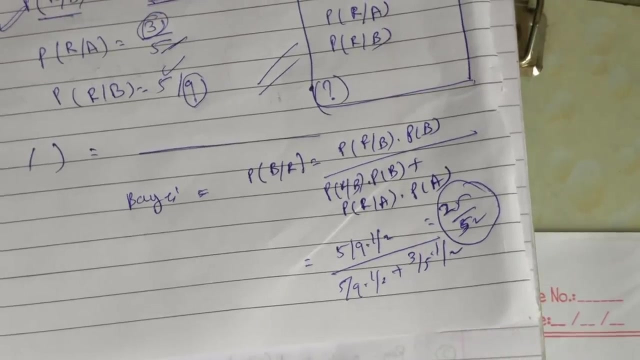 So answer would be twenty five by fifty two. So it was very simple. Just you need to know that first is normal probability and second is conditional probability and just check what is asked in the question and write and form something like this: you know this.